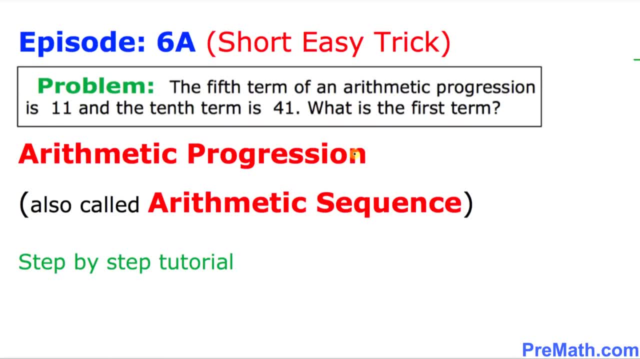 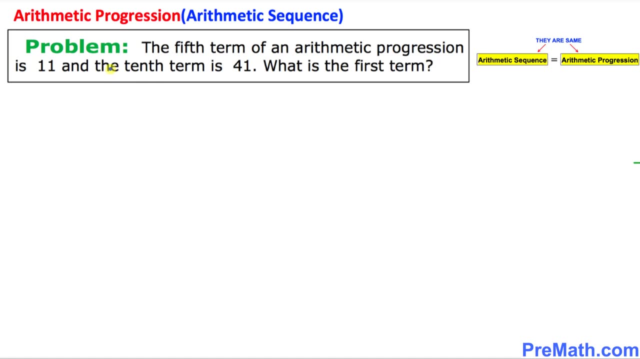 Welcome to PreMath. In this video tutorial we will be using this short and easy math trick on these arithmetic progression, or sometimes we call it arithmetic sequence, for this given problem. And here is our problem over here. It states the fifth term of an arithmetic progression. 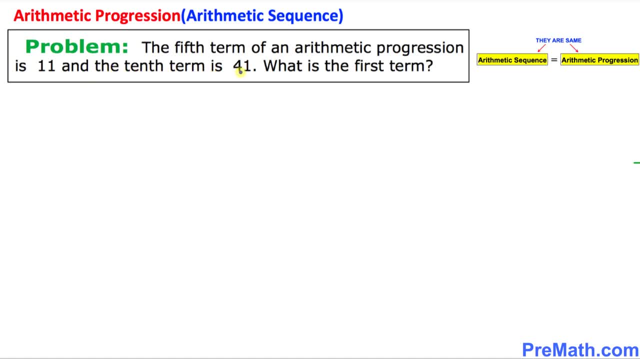 is 11 and the tenth term is 41. Find the first term. So what has been given to us? we know that a fifth term means a sub 5 equal to 11 and a sub 10 equals to 41. And we want to find the first. 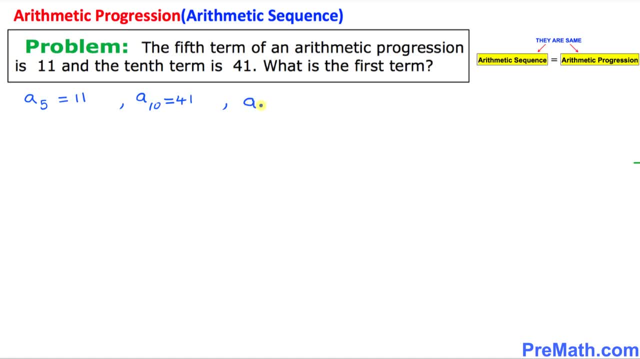 term. As I told you before, a sub 1 represents the first term. So we have this much given and this is what a sub 1 we want to find And in this very first step, we are going to find the common difference d, And we know that we have this much data given to us. 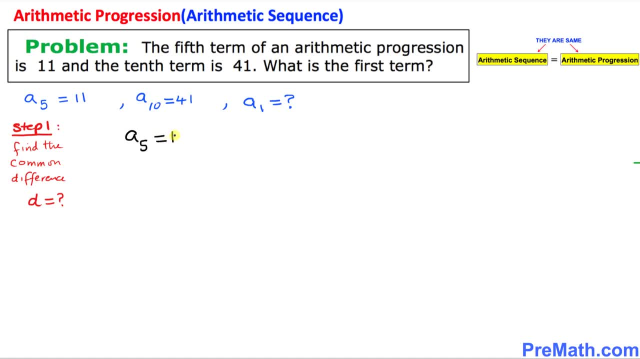 that a sub 5 equals to 11 and also a sub 10 equals to 41. from here, As you can see, this one, this has been given to us. I just wrote it down over here And here we will be using this. 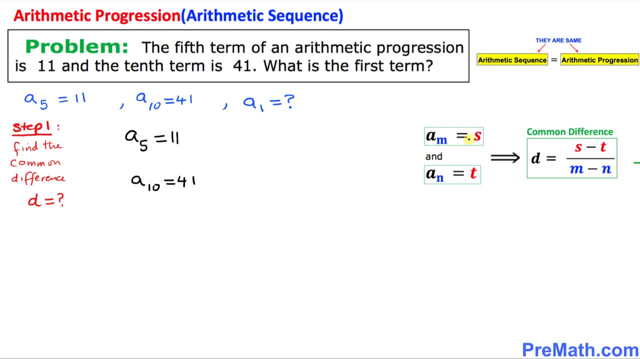 formula over here. As you can see, if I say a sub m equal to s and a sub n equals to t, just like this has been given to us, then the common difference is just the ratio of their differences. That means I can write this as: d common difference equals to: 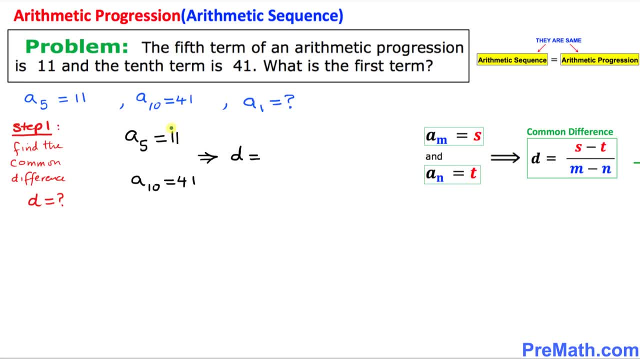 s and t. So I am going to write down these numbers. These are called s and t, 11 minus 41.. So I'm going to write 11 minus 41 on the top divided by likewise, I will be just putting: 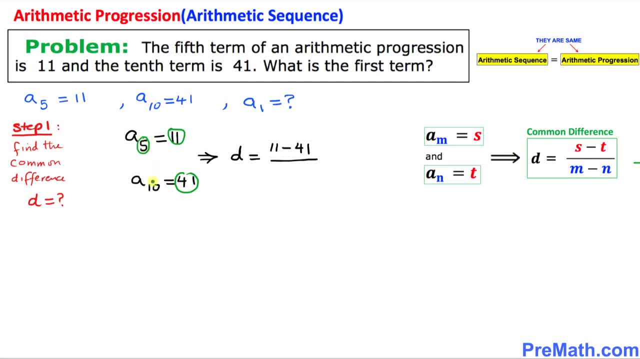 these numbers, these subscripts over here, So I can write 5 minus 41. And I can write 10.. That's pretty much it. And now let's go ahead and simplify this thing. So d is equal to. on the top it's going to be negative 30 over negative 5.. So d simply turns out to be positive. 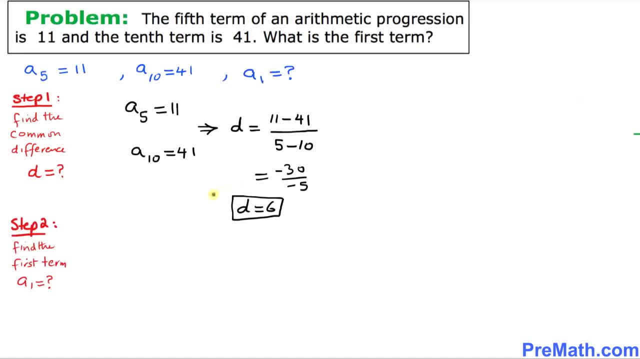 6. That's our common difference. And now, in the second step, we are going to find the first term, which is a sub 1.. We want to find out To find a sub 1, we are going to find out. 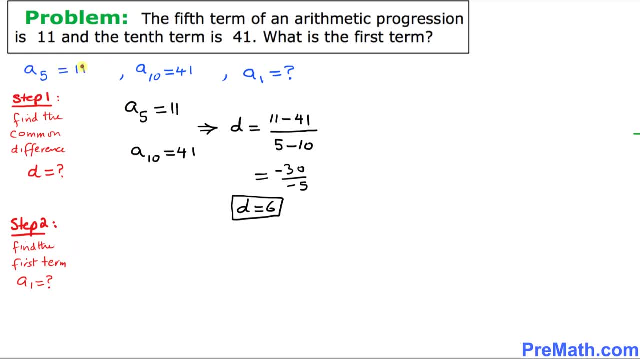 a sub 1.. The very first thing we are going to do is we have these two things been given to us: a sub 5 equal to 11 and a sub 10 equal to 41. We want to pick the easy point, So. 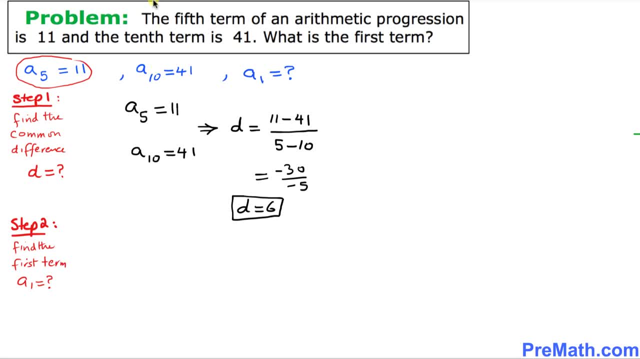 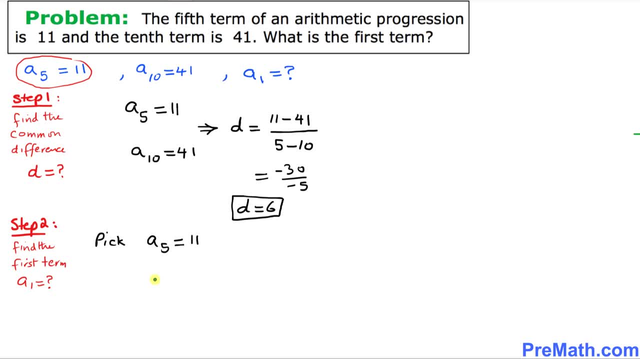 a sub 5 equal to a sub 5 equal to 11.. Now, as you can see over here, the subscript over here is five. That means that tells us that our n equal to 5.. And now we are going to use this arithmetic. 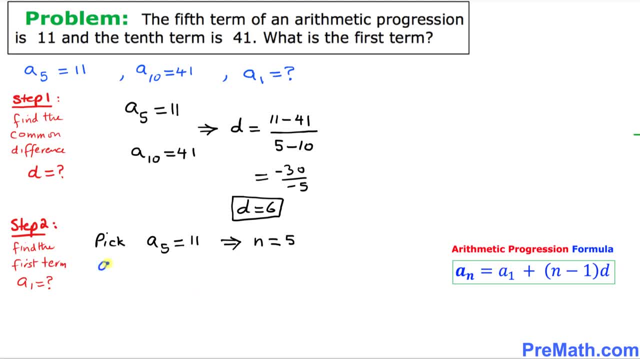 progression formula. Let me write it down over here: As of n equal to a sub 1, plus n, minus 1.. times d: and here we are going to write down over here a sub n, in our case is a sub 5. i'm going to. 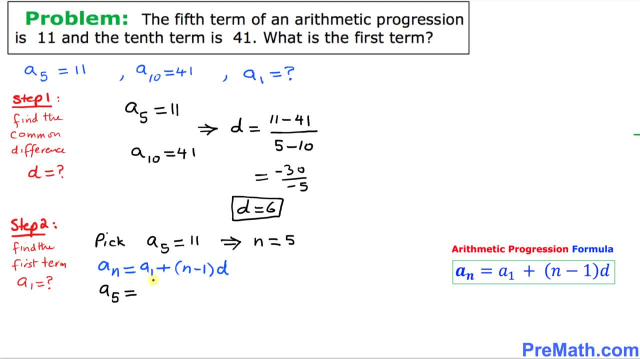 write down a sub 5. we are in. we need to find a sub 1. just leave it that one plus from our- this case n is 5 and you can see 5 minus 1 times d. in the previous step we figured out d equal to. 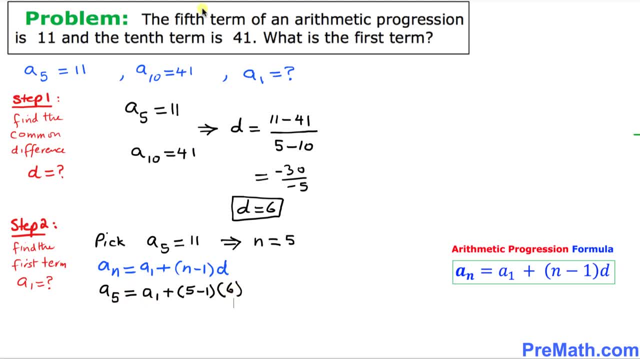 6, just write it down. let's simplify. we know that a sub 5 equal to- right up here- 11. you can see that one, so i can write: 11 equals to a sub 1, plus this simply become 4 times 6, let's simplify. furthermore, 11 equal to a sub 1 plus 24, let's move.